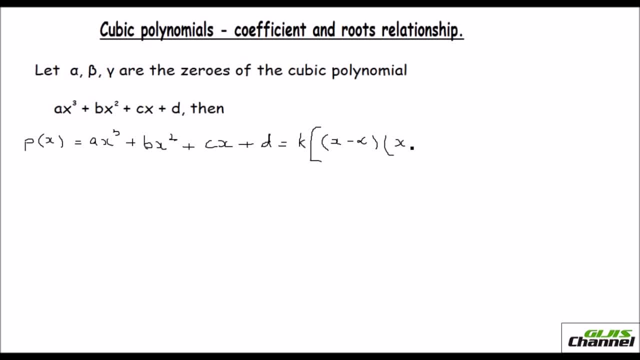 x minus beta as my second factor And x minus gamma as my third factor. okay, So it would be factorized and the result would be like this: right, So let us solve for this, to find the relationship between them. For this, what I do is I just still keep the k out. 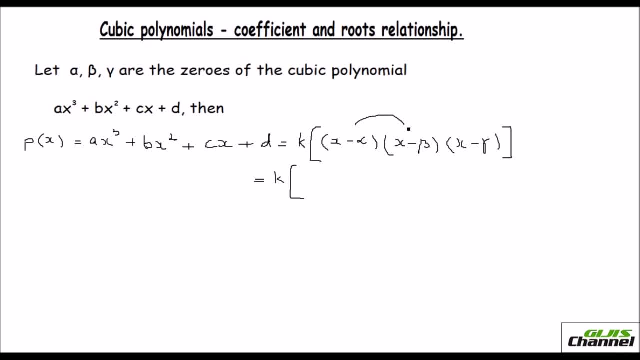 and I am going to multiply this and this. okay, These two factors, I am going to multiply and I am multiplying. So what happens? It would be x squared. FOIL it. okay, You know how to do the FOILing right: First terms first, then the outer terms. So that would. 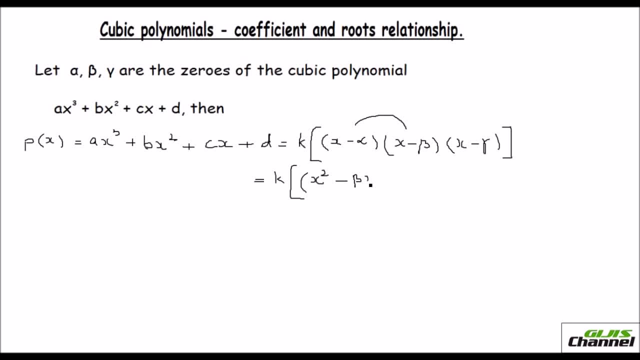 be minus beta, x, right. Then the inner terms: minus alpha, x it is. And then the last terms: so that would be plus, because minus alpha and minus beta will makes it plus, okay, And then you have this third factor here out. So let us do that now, So in the next. 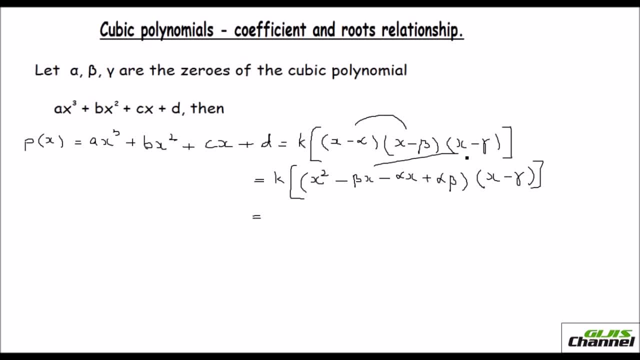 step. I am going to multiply these two. okay, These two okay. So what I do? and still, I keep the k out till I solve the factors, I mean till I multiply the factors. So what happens here? You would get x cubed minus gamma, x squared. 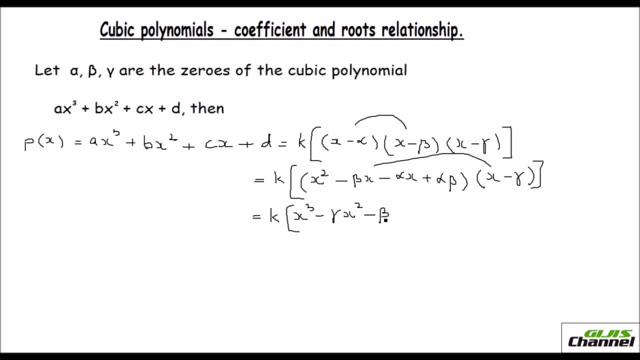 Minus beta x, squared plus gamma and beta x. okay, Now when I multiply with the minus alpha x, it would be minus alpha x squared plus alpha gamma x. Now I multiply with the alpha beta. okay, So that would be plus alpha beta x squared plus alpha gamma x. Now I multiply with the alpha beta. okay, So that would be plus alpha beta x squared plus alpha gamma x. Now I multiply with the alpha beta. okay, So that would be plus alpha beta x squared plus alpha gamma x. Now I multiply with the alpha beta. okay, So that would be plus alpha. 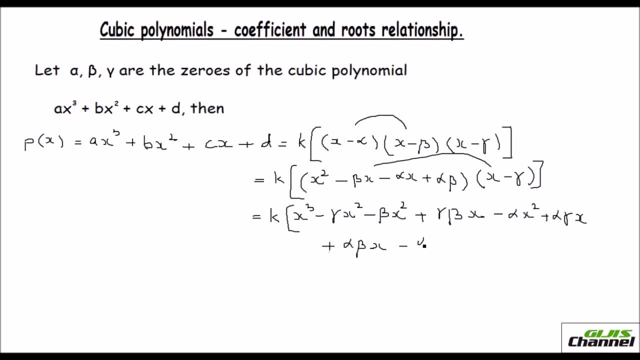 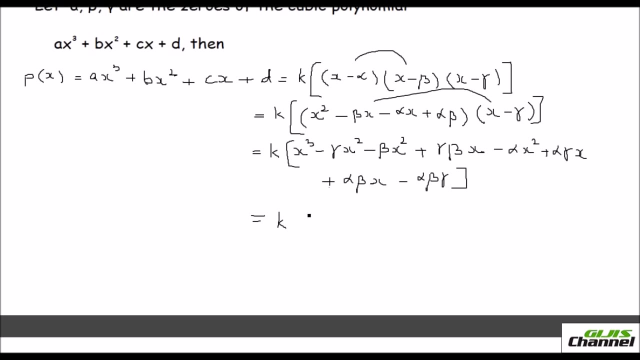 x minus the alpha, beta and gamma. okay, so I have just multiplied all the factors. next, let us put the like terms together, so that would be K times so X, cube. let it be together and let's put all the X squares out so you would get. I take the 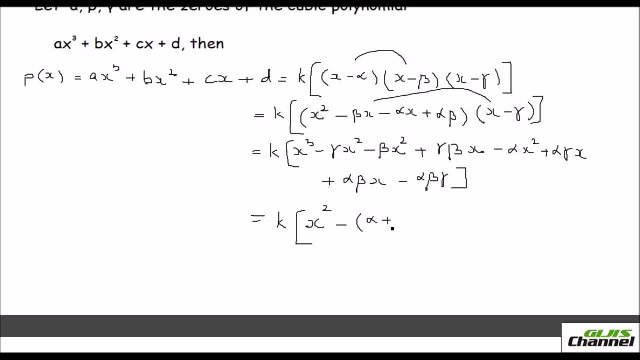 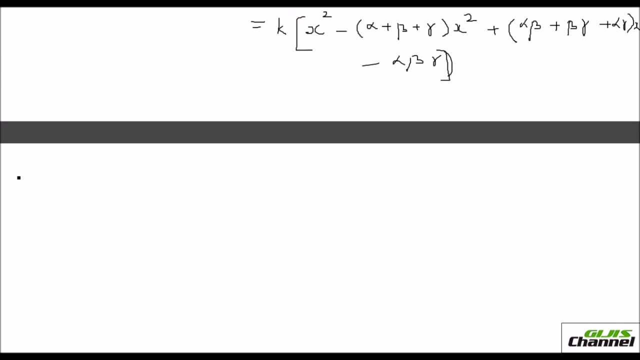 minus, sign out. so it will be alpha plus beta plus gamma x squared right now. taking the X terms out, that would be plus, and the X terms are like alpha, beta plus beta, gamma plus alpha, gamma, X minus, you have alpha, beta and gamma. okay, So finally you have got ax cubed plus bx squared cubic polynomial right plus cx plus d equals. take the k inside, so that would be kx squared minus k times. alpha plus beta plus gamma x squared plus k times. 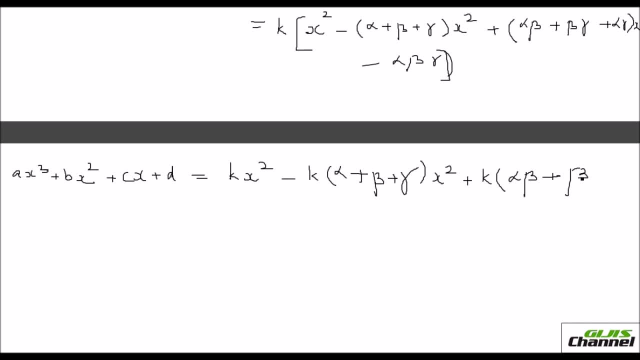 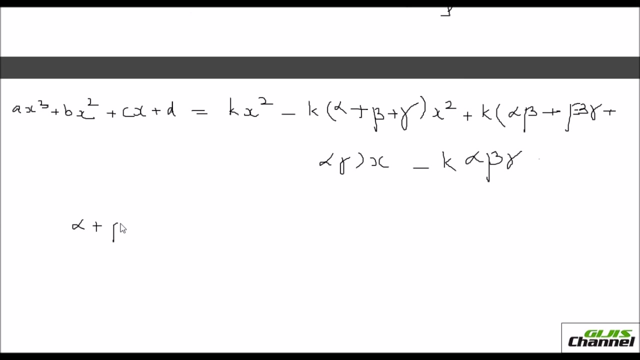 Alpha beta beta gamma plus alpha gamma x minus k alpha beta gamma. right now, let us equate it Now. what will your alpha Plus beta plus gamma b? it would be like: yeah, I've got minus k times x squared right. x squared is equal to bx squared. 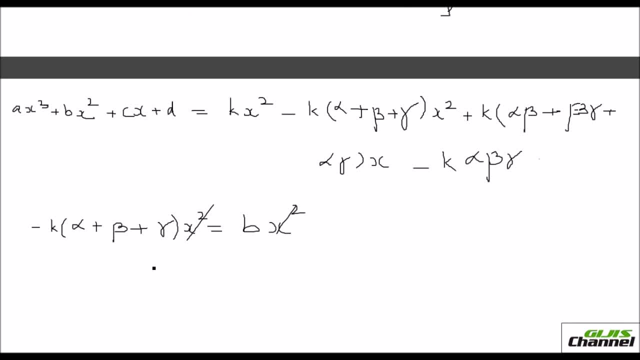 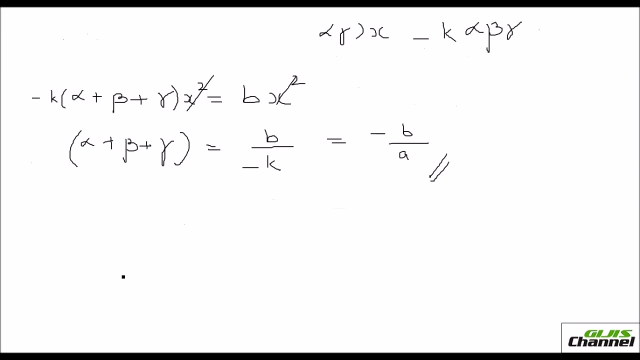 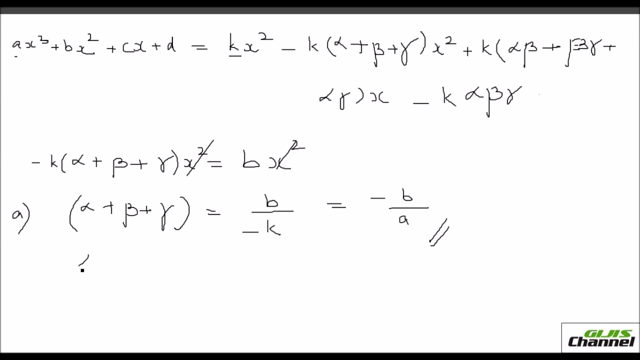 So, cancelling the x squared, what we have we have alpha plus beta plus gamma- is equal to b over minus k. You know that the K is equal to a, so k is equal to a. so I replace the k with a, so that will be minus b over a. okay, so you got your alpha plus beta plus gamma as a. so this one we have got now the second one, same way you're going to equate to the alpha plus b, alpha beta plus beta gamma. so I just write that. 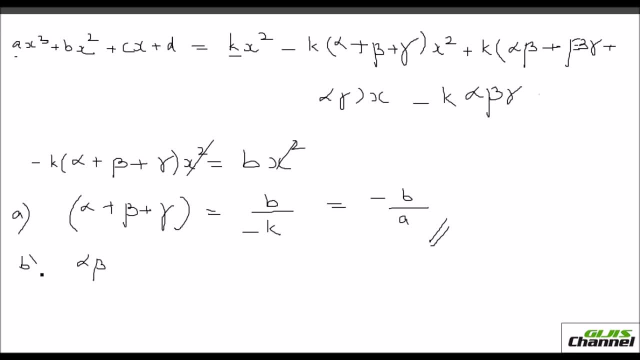 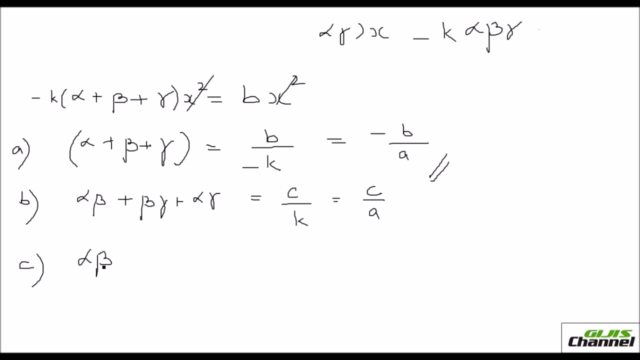 Straight away. The second thing you would get is alpha, beta plus beta gamma plus alpha gamma will be equal to c by k, so that is nothing but c over a, and finally You would have alpha, B, Beta And gamma. okay, alpha, beta and gamma. 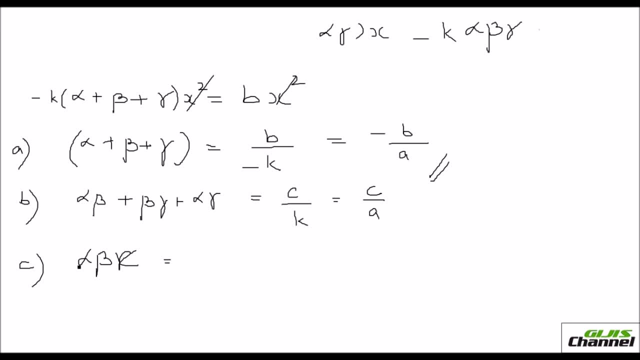 Will be equal to. This is Minus d over k. okay, That is nothing but Minus d Over a, Understood. so these are the three values. you have derived that, okay. so this is the relationship between A In a cubic polynomial, the relationship between the roots, alpha, beta, gamma and the coefficients minus b by a, c by a and. 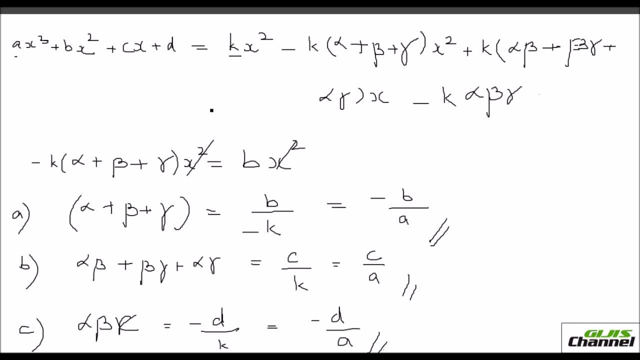 Minus d by a. okay, so this is how we write the equation. it is K x square minus k alpha plus beta plus gamma, the whole square Plus k alpha beta plus beta gamma, plus Alpha gamma. x Minus K alpha beta gamma. okay. 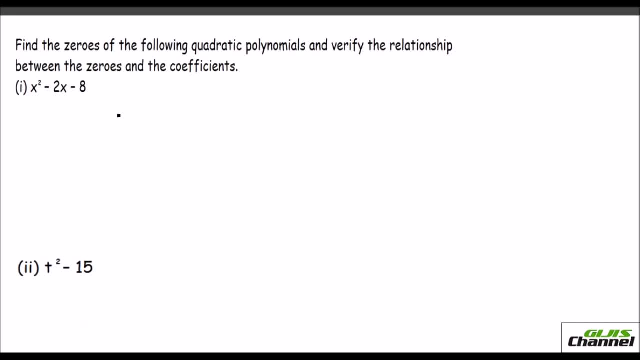 So let us put them in a problem. I have taken two Quadratic polynomial and a cubic polynomial. Here You need to find the zeros of the quadratic polynomial and also you should verify the relationship between the zero and coefficient. So let us first find the factors of this. 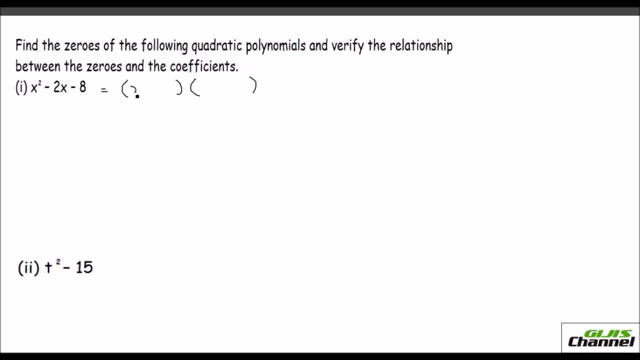 Quadratic polynomial right. So it is x And x here. So It should be like minus eight and Here it is minus two right, Negative eight and minus two. So what are the values you can take? Four and two right. 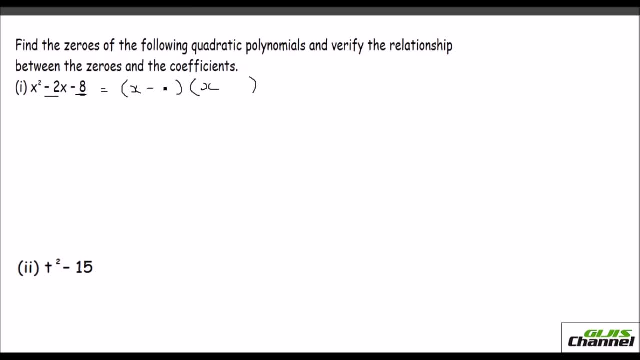 So let us take it as Minus four And plus two. So we got the factors here. Now let us write the relationships. So what are the roots here? So you get your roots as x equals Four Or Negative two. okay, 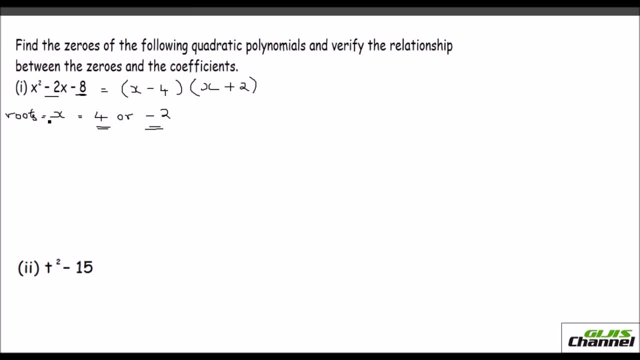 These are the roots now. So here you need to find the sum of the roots, That is alpha Plus beta. right, Alpha plus beta. What do you get? You get four Plus negative two, So that is a two. here The coefficient is: 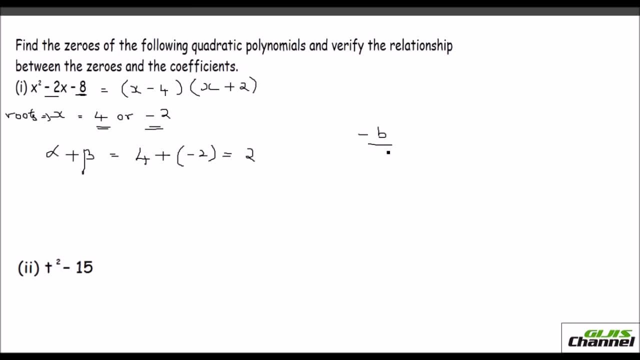 Minus b by a right. The sum of the roots should be minus b by a. Let us check with this equation Here: your a is one, Your b is Minus two and your c is Minus eight. Minus eight right. 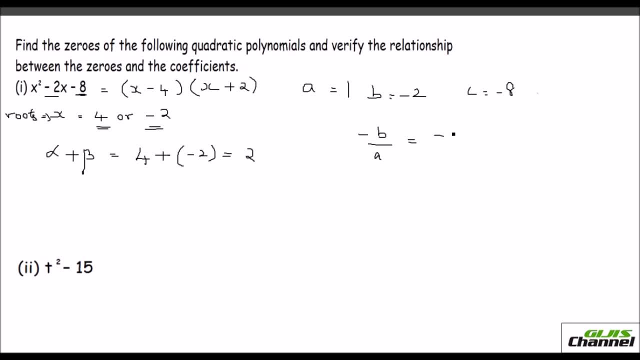 So let us What is minus b by a, So that is minus two over one. Minus of minus two- sorry, You have minus. side B is negative two. So minus of minus two will make it plus two. Okay, So you can verify these. 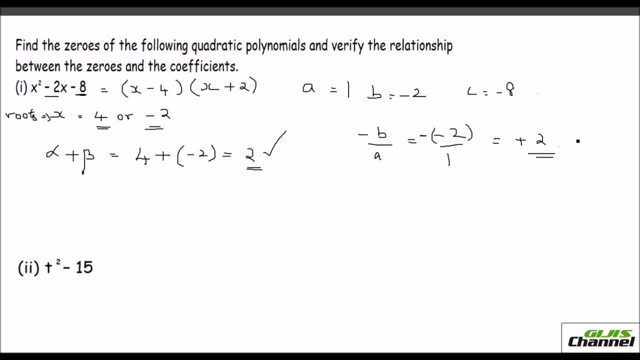 The sum of the two roots will be equal to Minus b by a. Okay, And now the product Alpha beta. You will multiply four times Negative two, right. So that will give you minus eight For alpha beta. it is. 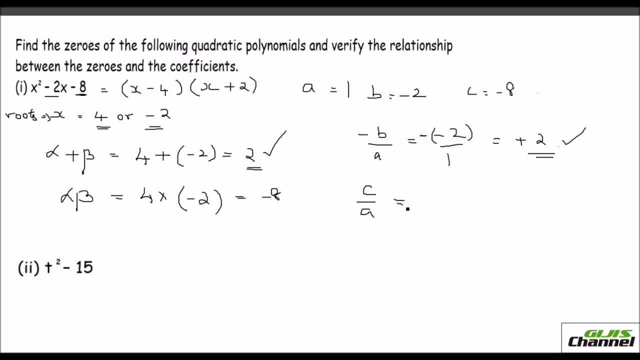 C over a right. So let us check that c. C is minus eight. Minus eight Over a is one. So you get minus eight. So you can find that these two are also same. So your product of the root will be equal to. 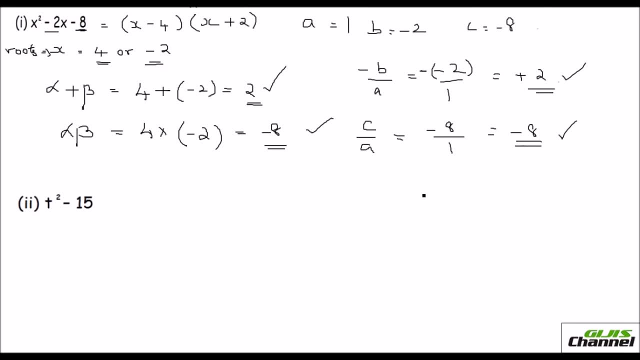 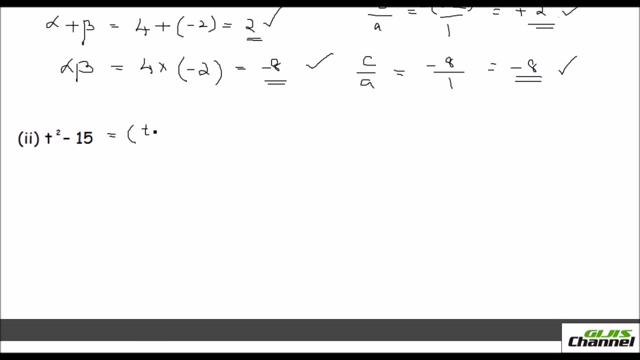 C over a Understood. I have taken another quadratic equation. So here again you need to factorize. So before factorizing I just change it. I rewrite it as T square minus Square root of fifteen, the whole square. So how do you factorize it?